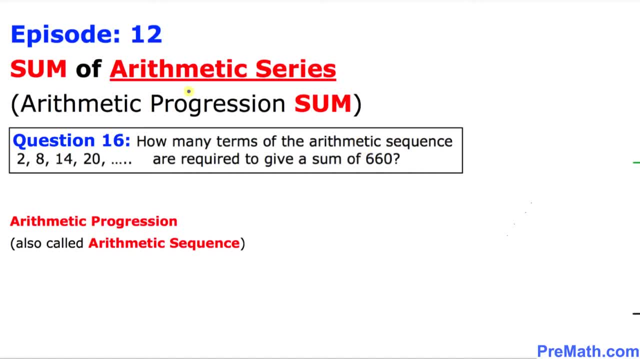 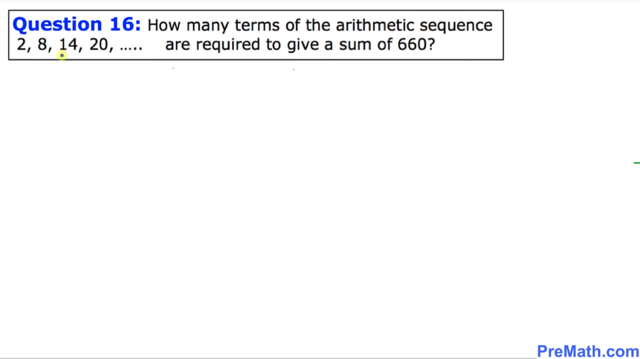 Welcome to PreMath. In this video tutorial, our topic is sum of arithmetic series and we will be taking care of this question as well. And here is our question: How many terms of the arithmetic sequence 2,, 8,, 14,, 20, and goes on and on, are required to give a sum of 660? In this case, 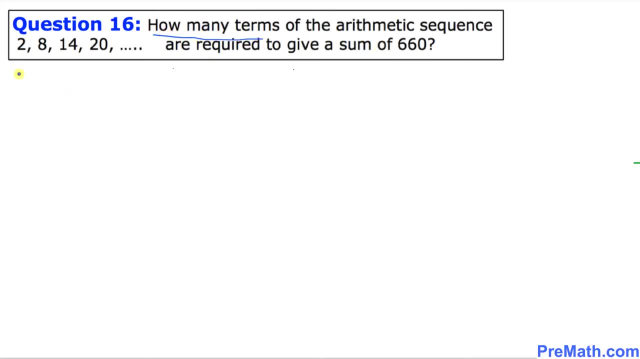 we are going to find the number of terms. That means we don't know n equals to how much, And we know that s of n, the sum of the terms, those terms is 660.. And, as you can see over here, our very first term: a sub 1 equal to 2. And one. 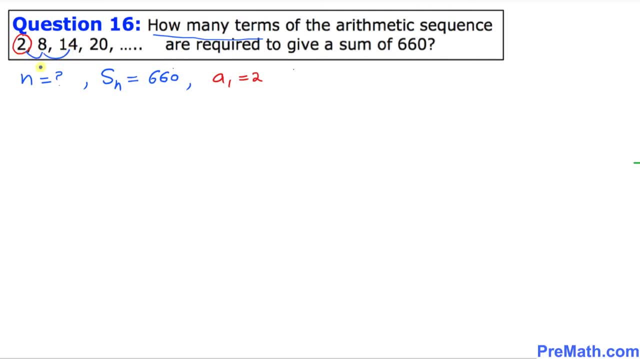 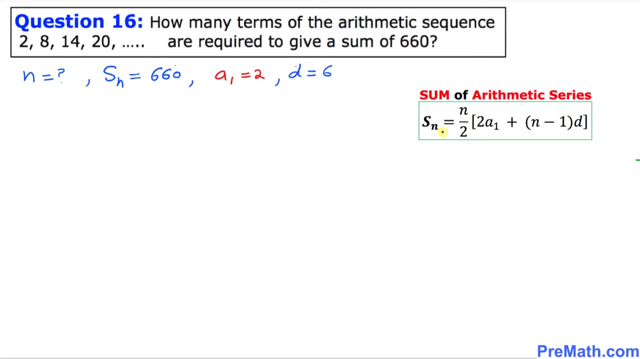 one more thing And our common difference. as you can see, if you add 6 to each term, we're going to get the next one, So d is going to be positive 6.. And here's the formula that we will be using now: Sum of the arithmetic series, and over here let me just put it down: S of n equals. 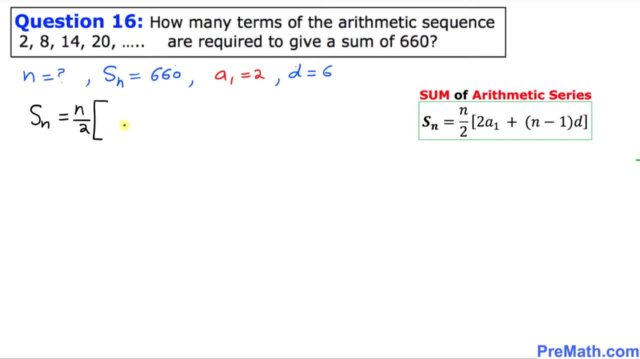 660.. We don't know n divided by 2.. And, inside parentheses, 2 times a1, in our case is 2 plus once again we don't know. n minus 1 times d, in our case, is 6.. Let's simplify this one, But we know. 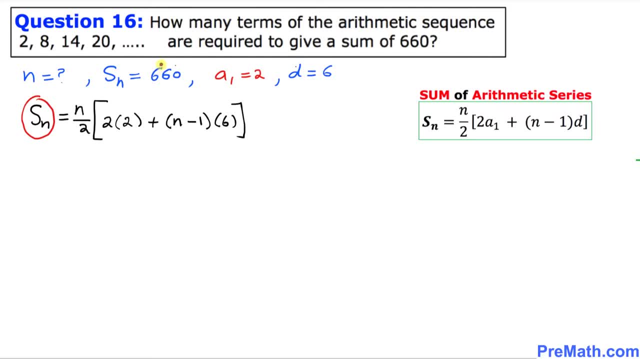 in our case, s of n is 660.. You can see this one, So I am going to replace this: s of n is 660, equal to n over 2.. And this 2 times 2 is going to become 4 plus if I distribute this, 6. 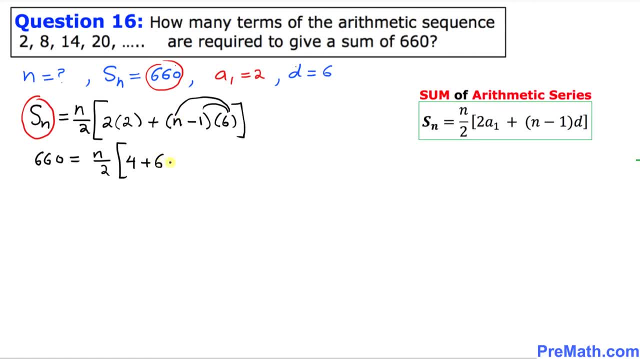 with both of these terms, that's going to give us 6n minus 6.. Let's simplify. furthermore, That's going to be n over 2. And this is going to be 4 minus 6. It's going to give us negative 2.. So I can write 6n minus 2.. And here, once again, I can do n over. 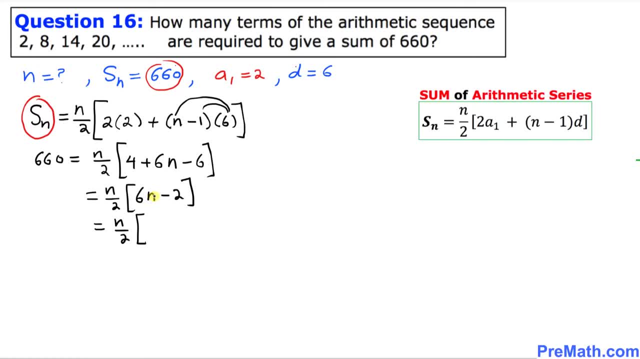 2. And here, inside this bracket, 2 is in common. I can factor it out. It could be written as 3n minus 1. And here this 2 and this 2 cancels out. So simply, we got 660. 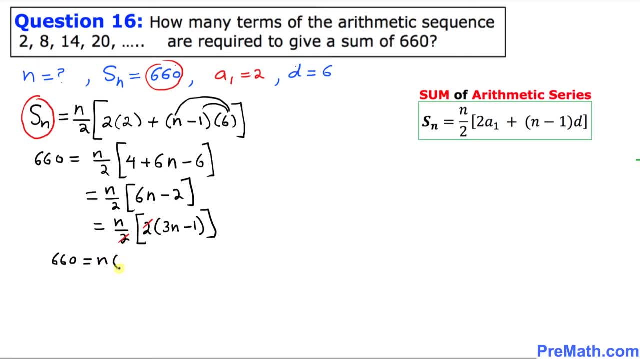 equal to n times 3n minus 1.. Let's go ahead and distribute this n with both of these terms. So we got 660 equal to 3n square minus n. And let's move this 660 on the right-hand side. So we got 660 equal to 3n minus 1.. And here this 2 and this 2 cancels out, So we got 660 equal to 3n minus 1.. And here this 2 and this 2 cancels out, So we got 660 equal to 3n minus 1.. And 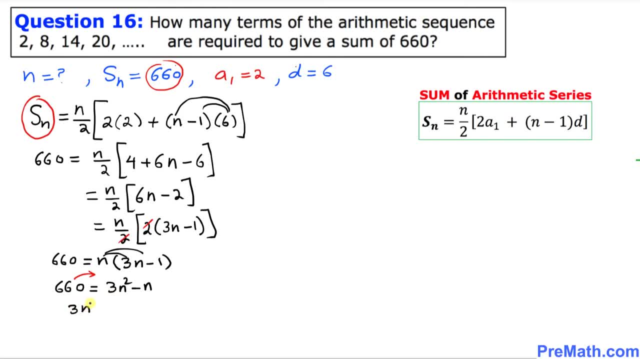 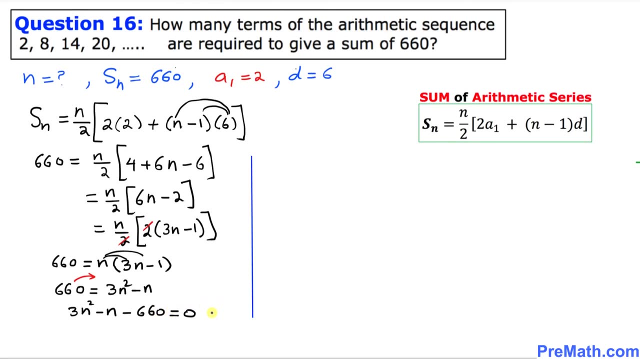 write this one as 3n square minus n, And this 660, when you go on the other side, becomes negative 660, equal to 0.. And now, since we are running out of space, I'm going to move over here. So this: 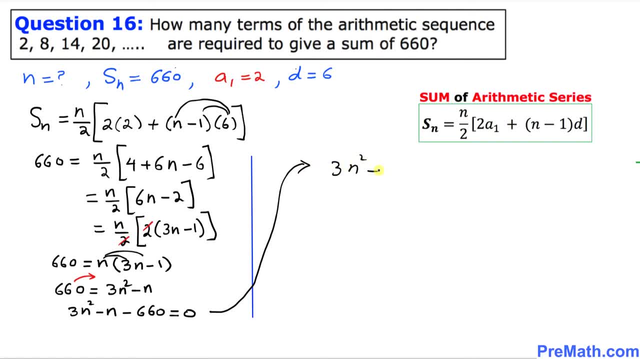 3n square. I'm going to write down 3n square minus 1n minus 660.. equal to 0, and here I can. this is a quadratic equation, I can easily factor it out and the possible factors are going to be: we can figure it out. it's going to be n minus 15 and the other one 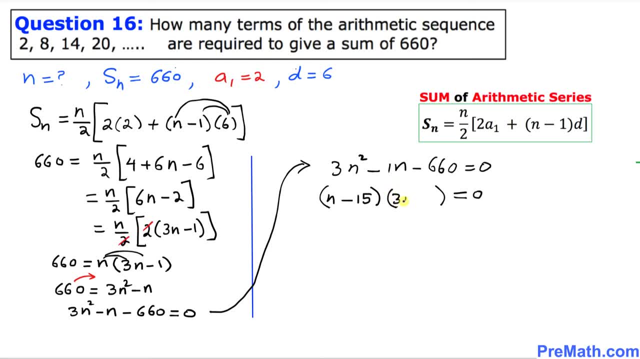 is 3n plus 44, all right. and now so n minus 15 times 3n plus 44, and since these two factors equal to 0, I can split them up, I can separate them, I can say n minus 15, equal to 0, and the